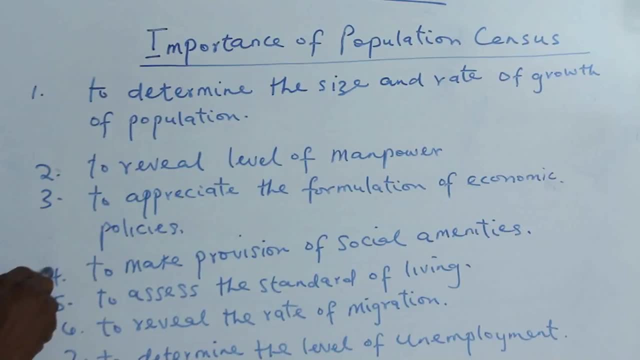 to know how to provide for social amenities in an economy or in a particular area of the country. Five, to assess social performs, The amount of money accepted from the economy during 80s, 60s, late 60s and the Laurie Clark you. Five, to figure out the extent of the economic. 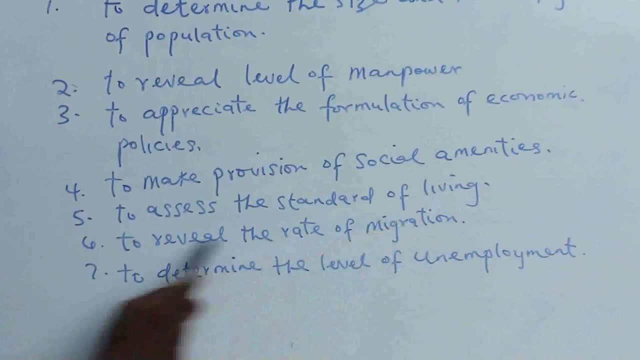 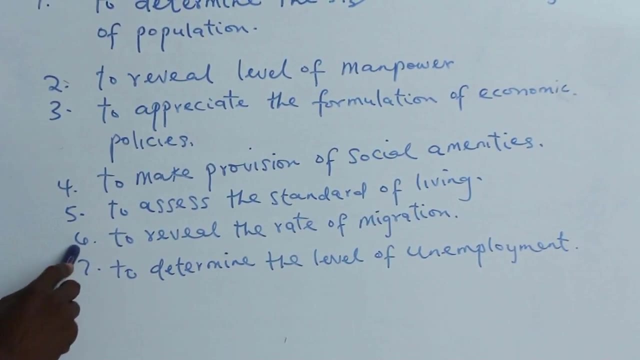 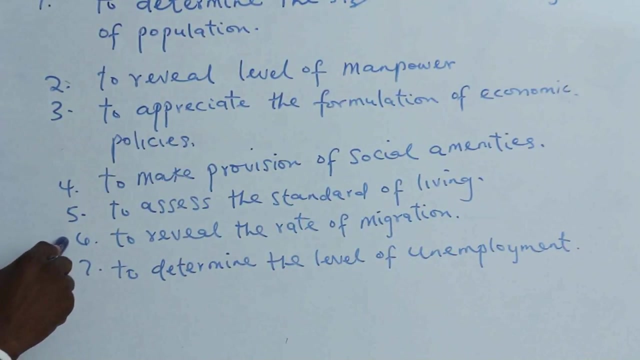 the standard of living. In knowing the standard of living with the help of population census, this can be known. Sixth, to reveal the rate of migration, That is to say how people are coming in into the country and how people are going out of the country With the help 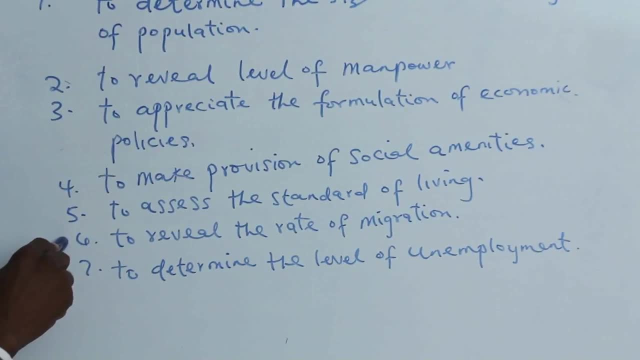 of population census. this can let the government understand how it is. Number seven: to determine the level of unemployment. I will carry out population census. This will reveal the number of people that are working and people that are unemployed in an economy. Problems of population. 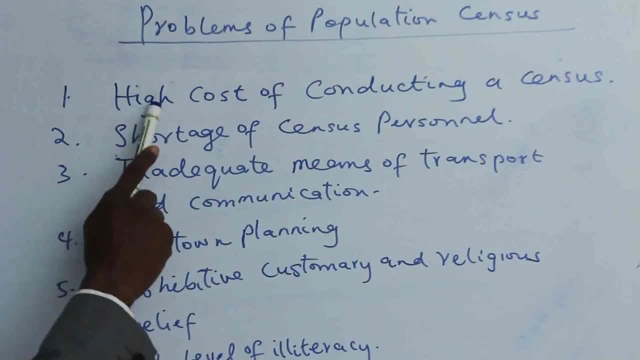 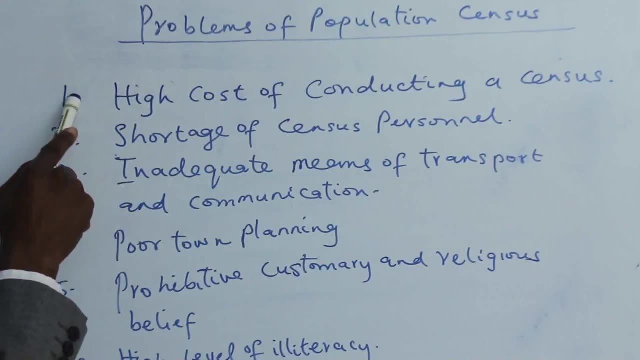 census. Number one: high cost of conducting a census. This is a problem. Many developing countries find it difficult to allocate funds into this program every 10 years. In that case, if they cannot do that, they won't be able to have or understand. 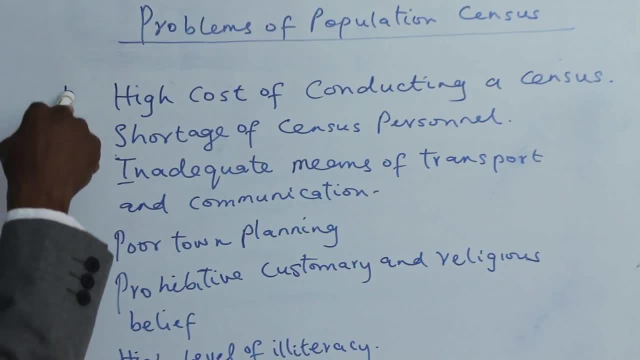 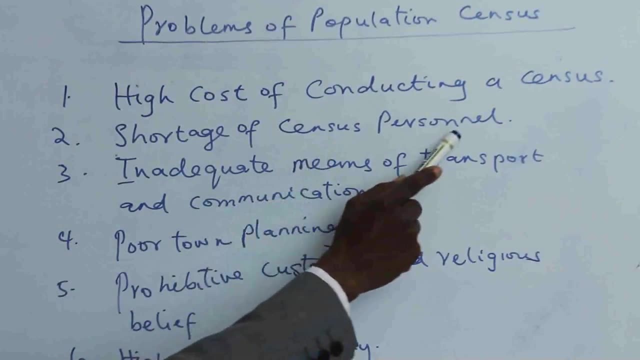 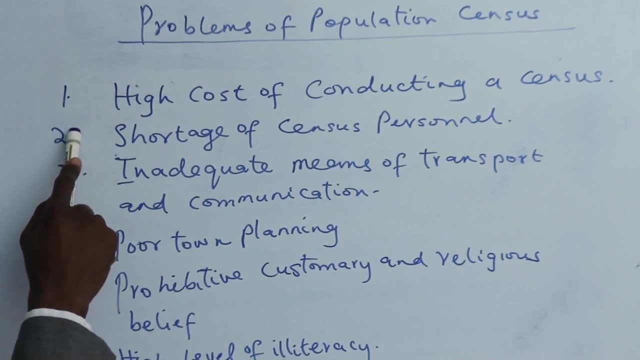 the population of the country. In such case it leads to a problem Number two: shortage of census personnel. In conducting population census, they need to have enough personnel that will handle the program. In developing countries they fail to have adequate personnel. 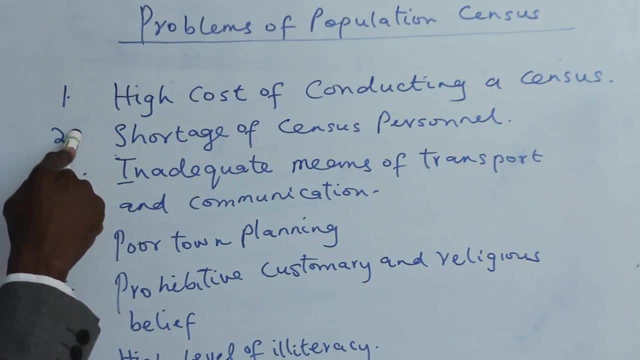 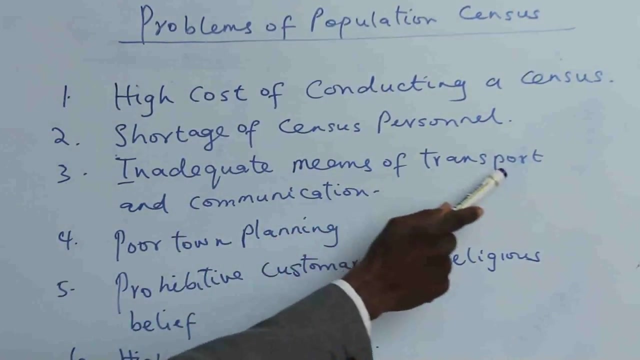 to handle the program, A situation where they are not able to get to the remote area. In such case it will become a problem when they are conducting a census. Number three: inadequate means of transport and communication, In the sense that in conducting a census, 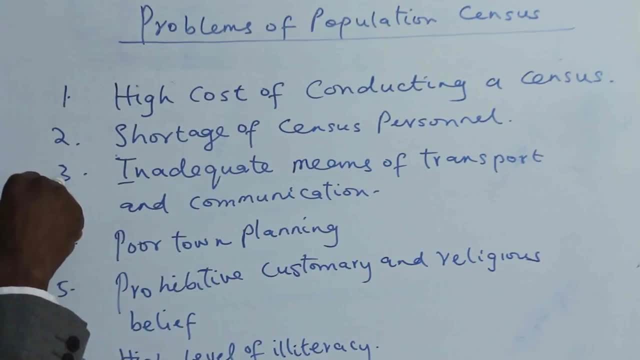 they need to have good road as well as good communication devices, But in situations where all these are not available, the personnel- the available personnel- will find it difficult to get to the remote area in order to carry out the census, as well as inadequate devices that 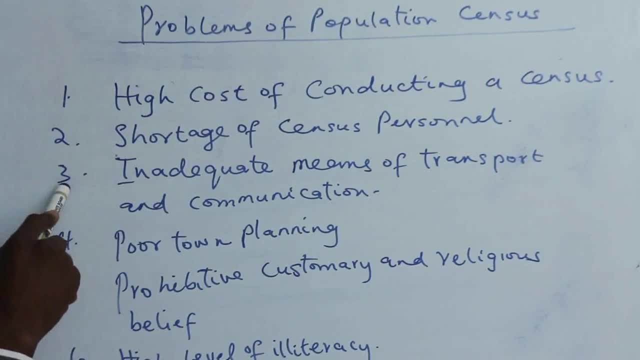 they can use that are not on-ground. They find it difficult to do that. Number four: poor town planning. Poor town planning is a problem in the sense that villages and towns are not well planned in terms of their buildings, in terms of streets having. 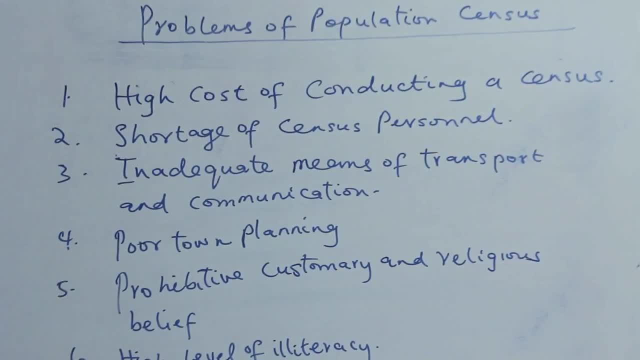 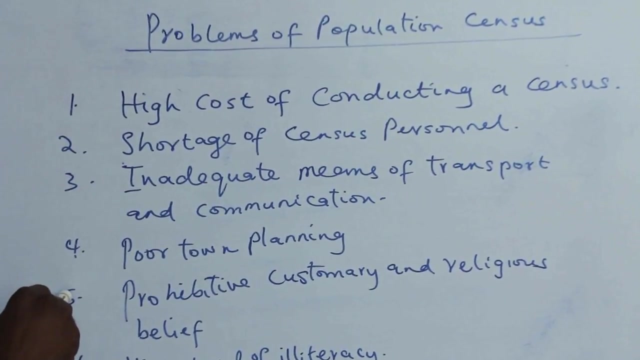 numbers and so on and so forth. Number five: prohibitive customary and religious belief In developing countries. they have a lot of custom To them. they don't believe in counting To them. they believe that by counting their children or their household. 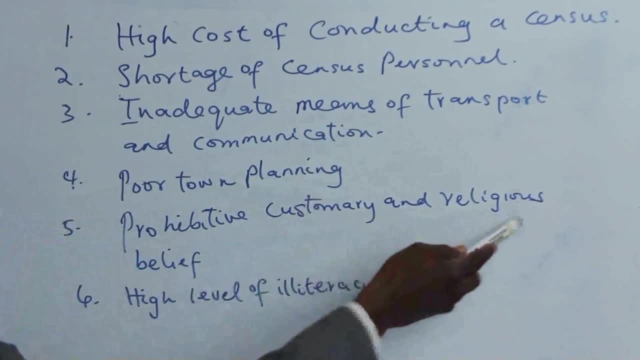 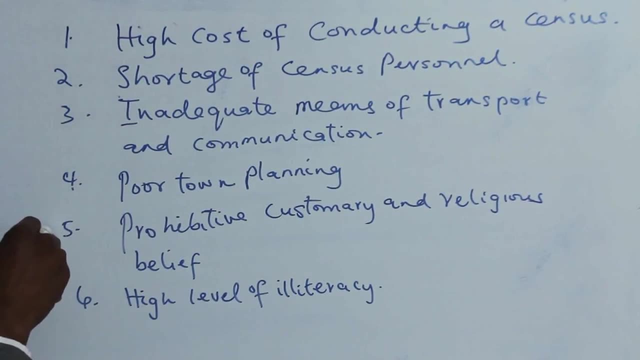 something will happen to them in the future, While, in terms of religion, Muslims believe that women are not allowed to be seen by men. So in that case, if we have male officials counting female households, there will be problems in that area. So, at the end of the day, they won't be able. 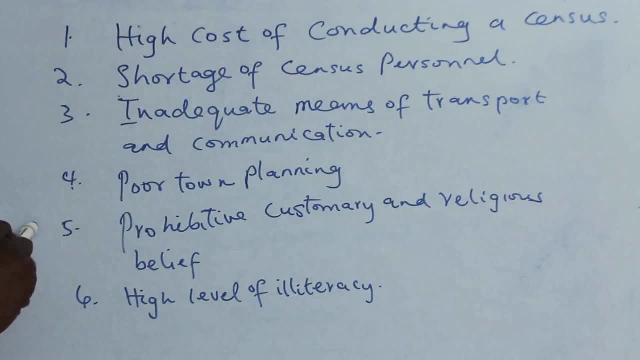 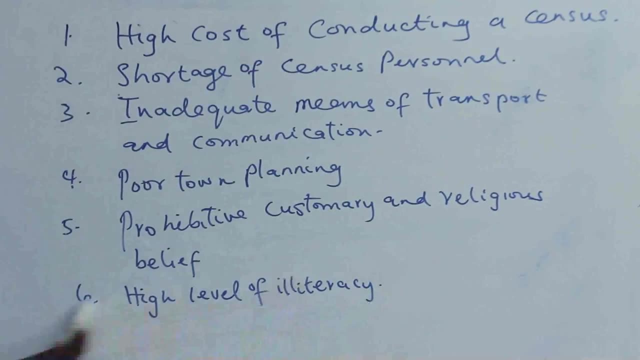 to count accurately. So it becomes a problem when they are having population censors. Number six: high level of illiteracy, in the sense that people don't disclose the fact before the official for them to understand. So at the end of the program the commission won't be able. 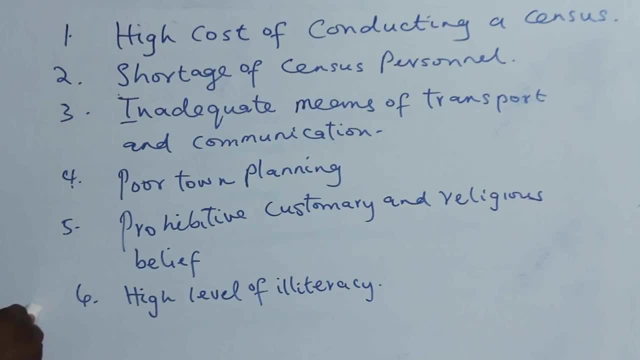 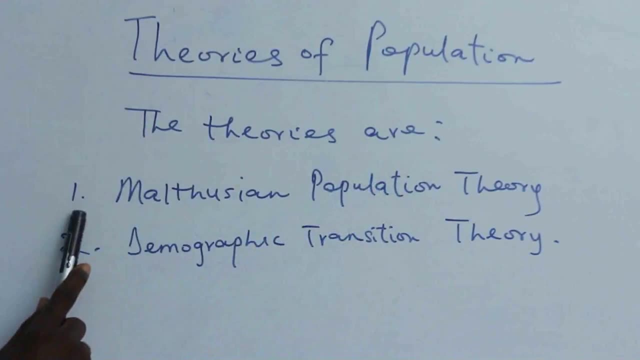 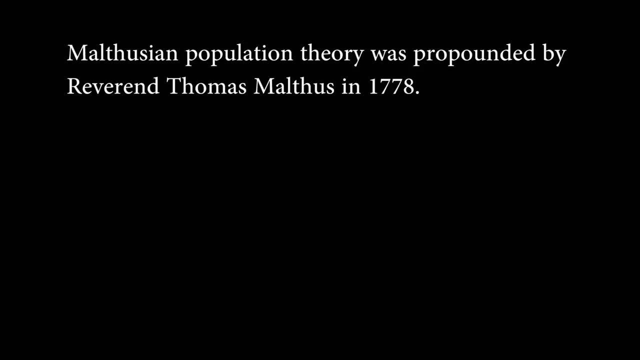 to reveal adequate information before the nation. Theories of population. The theories are one: Matosian population theory. Two, demographic transition population. Matosian population theory was propounded by Reverend Thomas Matos in 1778.. He was a well-known. 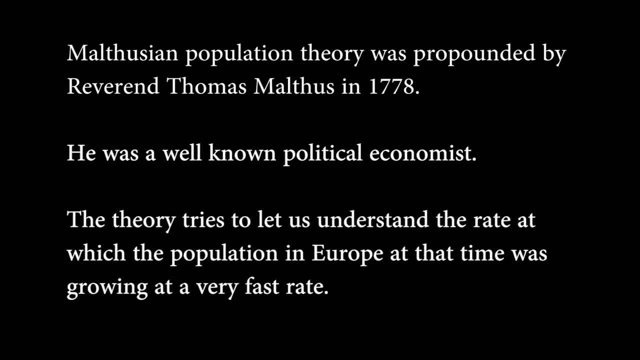 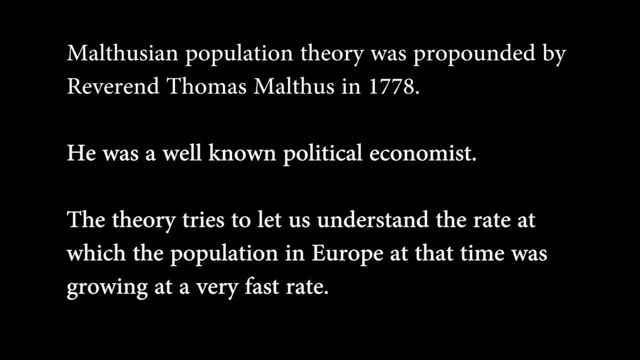 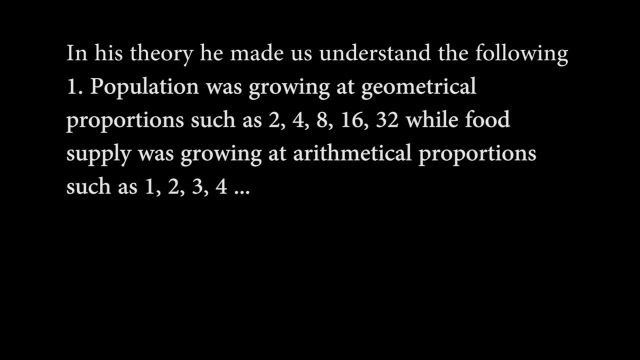 political economist. The essay, that is, the theory, is trying to let us understand the rate at which population in Eru at that time was growing at a very fast rate. In this theory he made us to understand the following One: that population was: 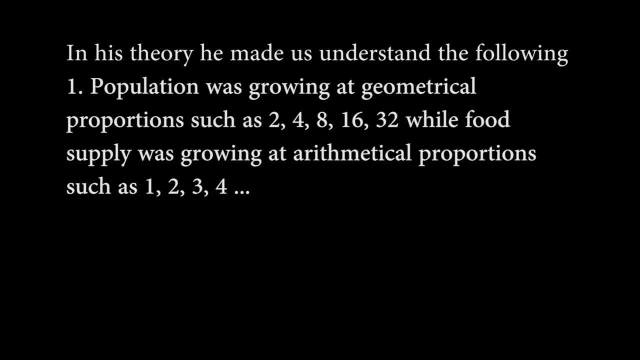 growing at a geometric proportion, such as 2,, 4,, 8,, 16,, 32.. While food production or supply was growing at arithmetical progression, such as 1,, 2,, 3,, 4, and so on and so. 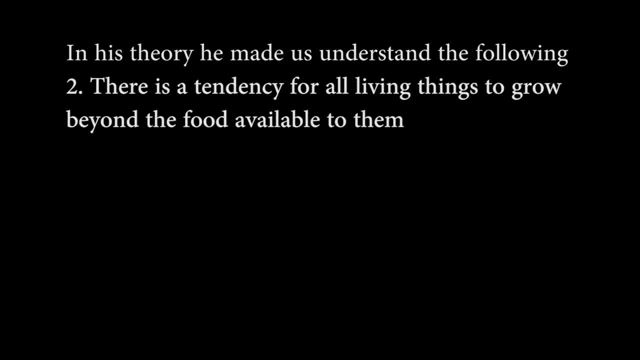 forth. Two, that there is a tendency for all living things to grow beyond food available to them. Three, that population is essentially limited, limited by the means of subsistence. Four, that unless population increase is matched with means of subsistence, 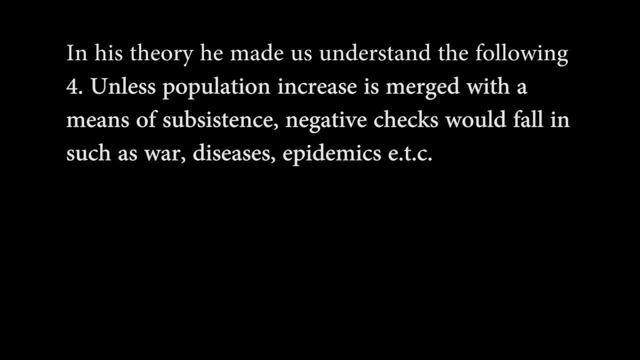 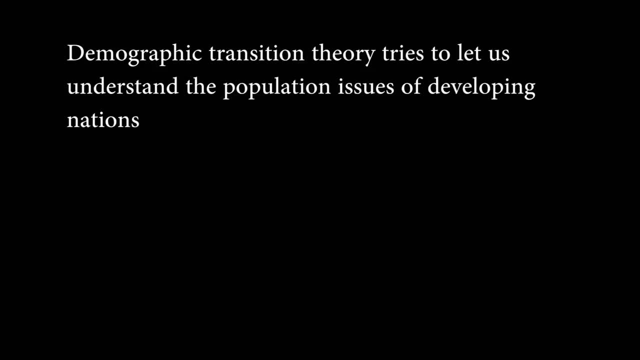 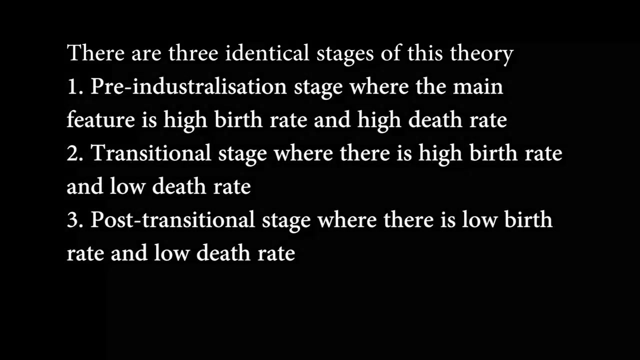 negative change will fall in, such as war, diseases, epidemics, etc. Demographic transition theory tried to let us understand historical explanation into population issues of developing nations, The three identical stages of this theory. One pre-industrialization stage. 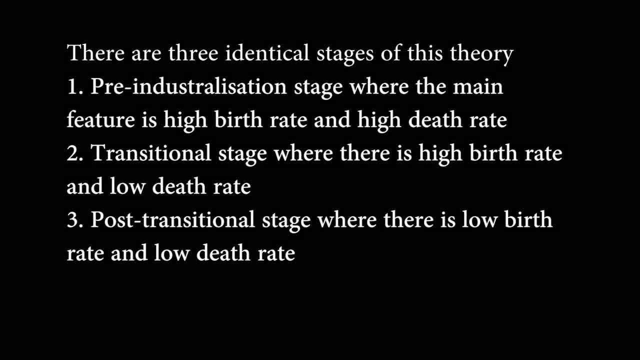 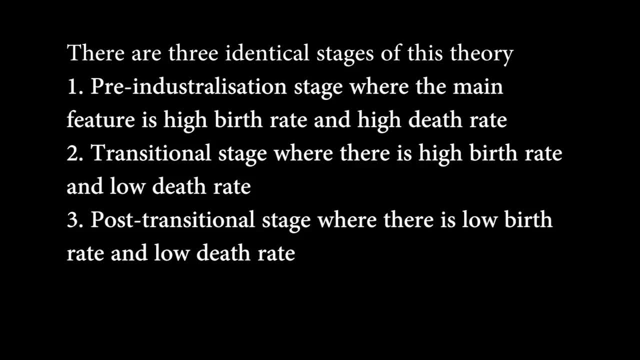 where the main feature is high birth rate and high death rate, That is, there is either static or increasing or decreasing at a lower rate in terms of population. Stage two- transitional stage- is characterized by high birth rate accompanied by low death rate. 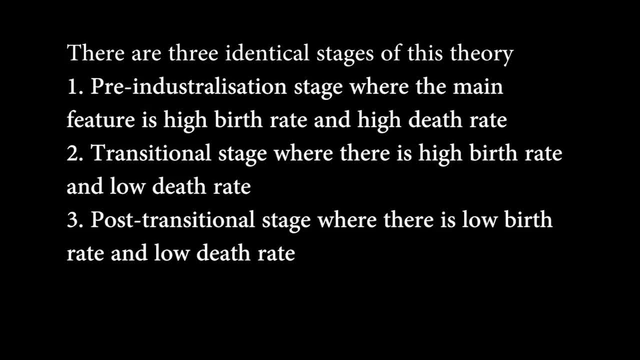 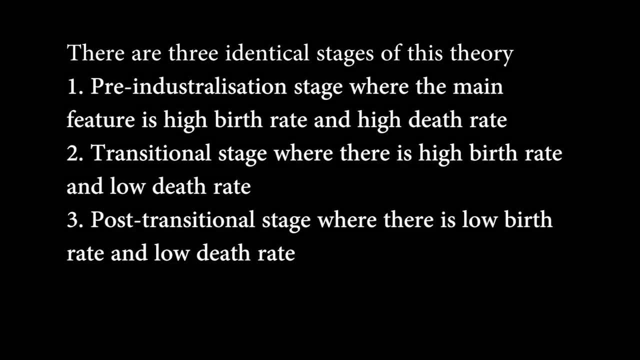 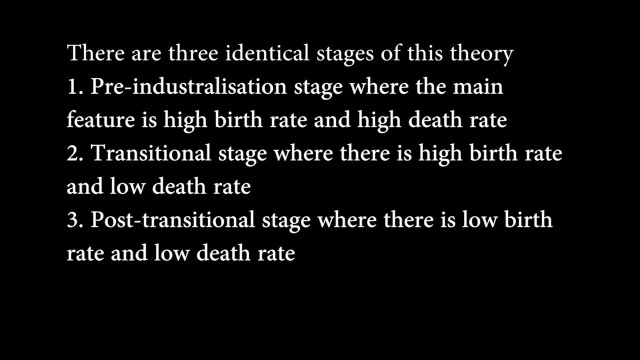 leading high population due to industrialization. better diet, improved medical services. This is associated with developing nations. Stage three- post-transitional stage. This is characterized by a low birth rate and low death rate, leading to little or no population growth. It is associated with advanced. 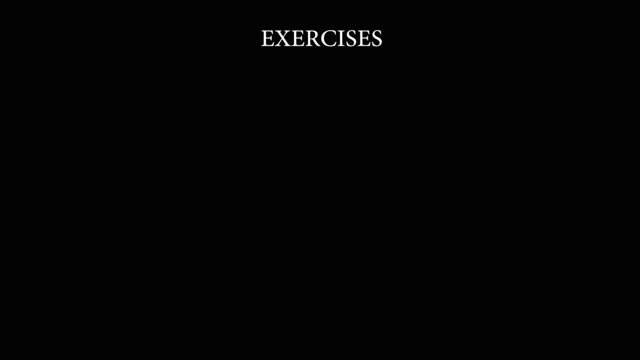 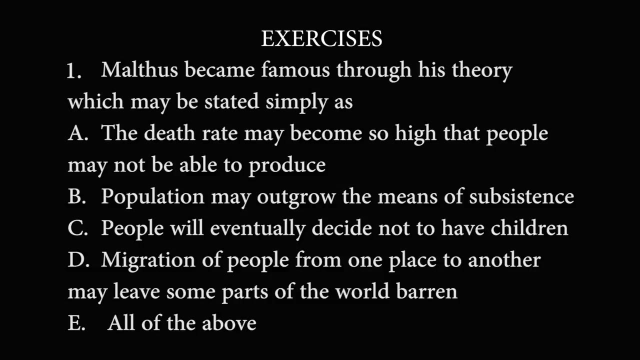 or developed countries. Exercises Question one. Matters became famous through its theory, which may be stated simply: A. the death rate may become so high that people may not be able to produce. B. population may also be able to produce. B population may also be able to produce. 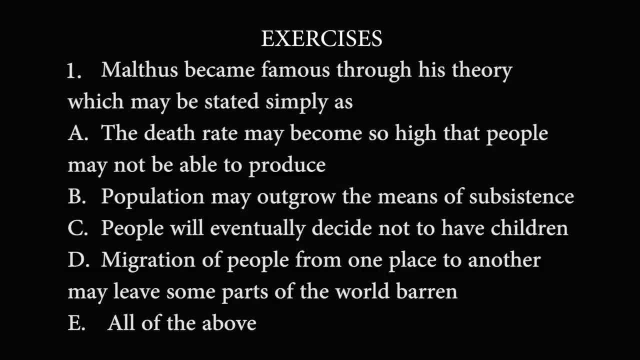 C population may also be able to produce. D. the population may outgrow the means of subsistence. C people will eventually decide not to have children. D. migration of people from one place to another may leave some parts of the world barrack.